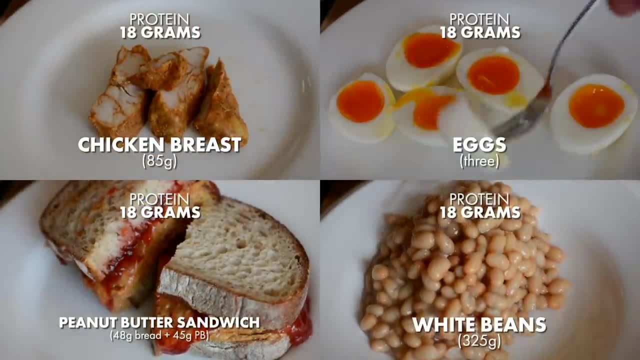 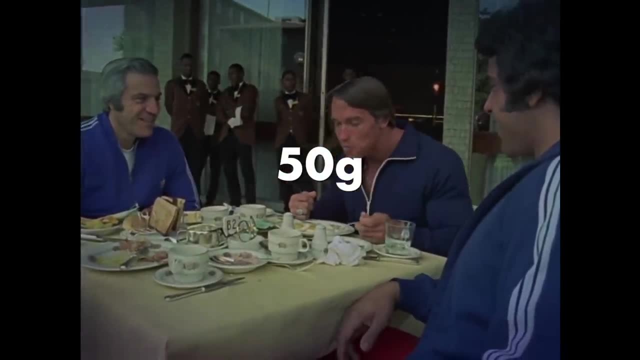 18 grams of protein from lentils or a peanut butter sandwich or some eggs. But here's something you might find surprising: 50 grams of protein per day is the minimum protein requirement for adults And if you look here, most of these 103 countries get most of their protein from plants, and they're 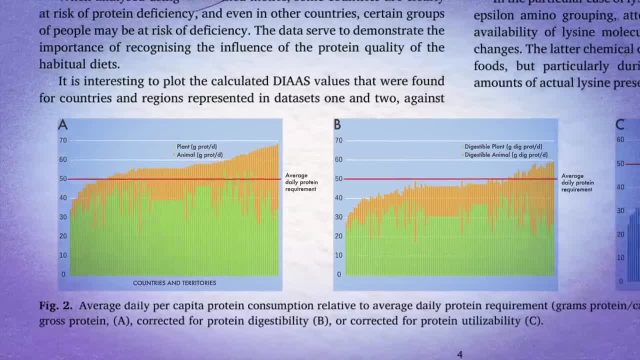 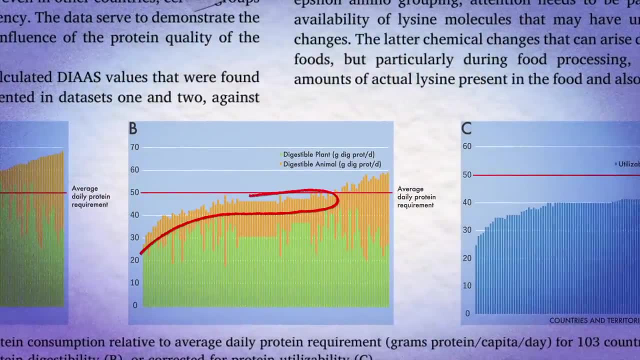 hitting their 50 grams a day. just fine, But plant proteins aren't digested as well. So if you incorporate the digestibility of the proteins, far more countries are just under the 50 gram requirement. Now, if you account for the fact that many plant proteins don't provide enough of one or 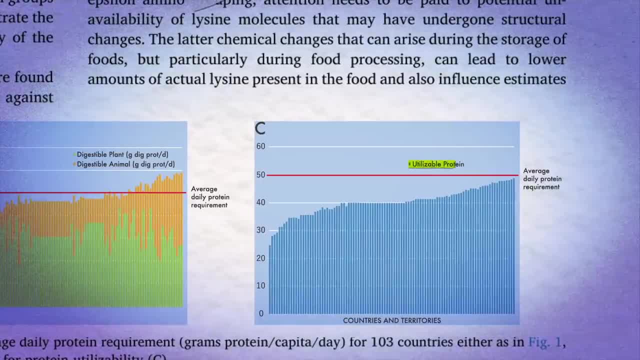 more of the essential amino acids. plant protein powders are just under the 50 gram requirement And therefore that protein can't be fully utilized. then it turns out that none of these 103 countries are hitting the 50 gram protein requirement. Now these countries could certainly. 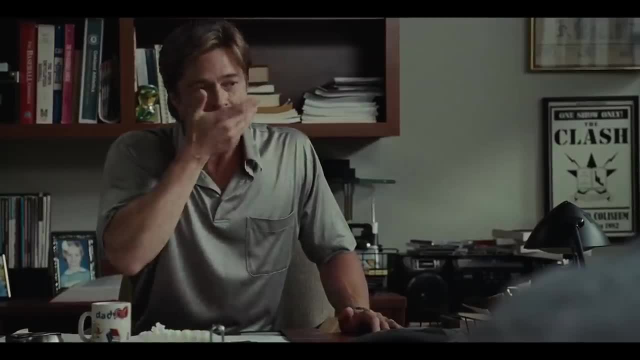 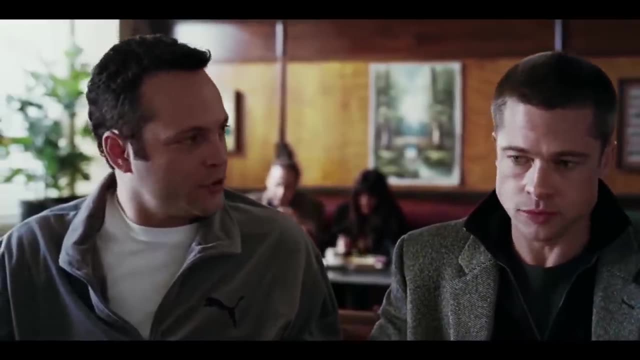 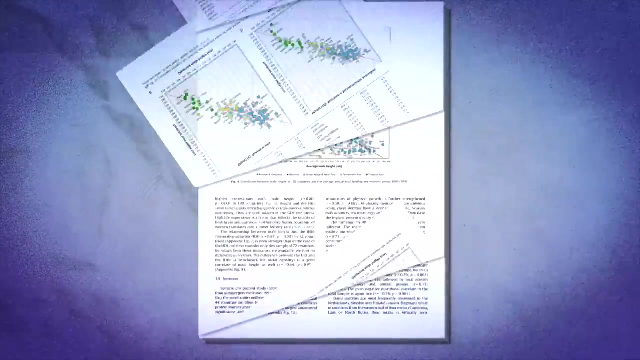 hit 50 grams of utilizable protein by simply eating a lot more plant protein. In developed countries we simply eat a bunch of protein in total, so this is less of an issue. But research suggests that protein quality may still matter. In a study looking at height of men in 105 countries, 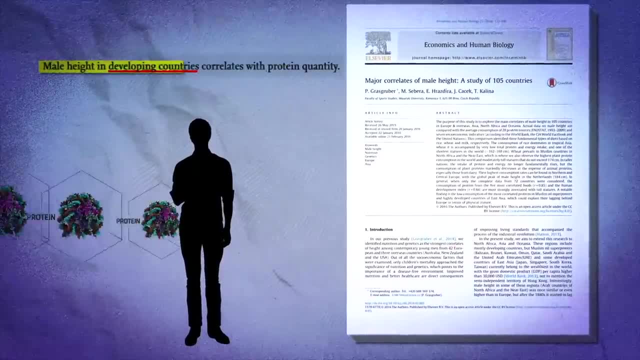 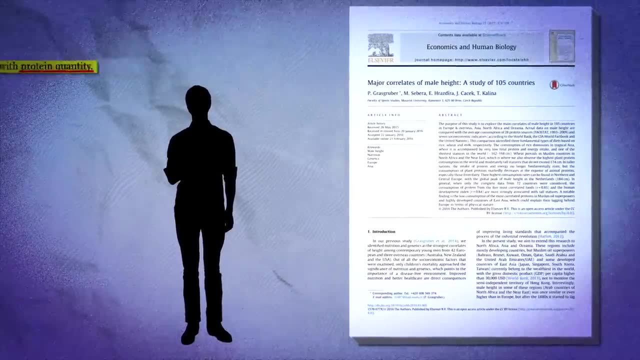 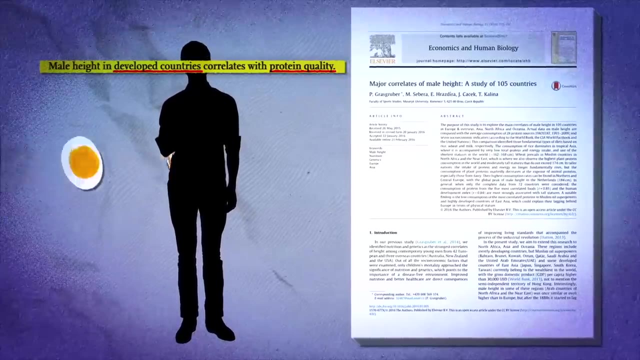 the height of men correlated with protein quantity. Unsurprisingly, the challenge in developing countries is having access to enough protein. However, in developed countries, where people eat plenty of protein, the quality of the protein they were eating is what mattered for height. 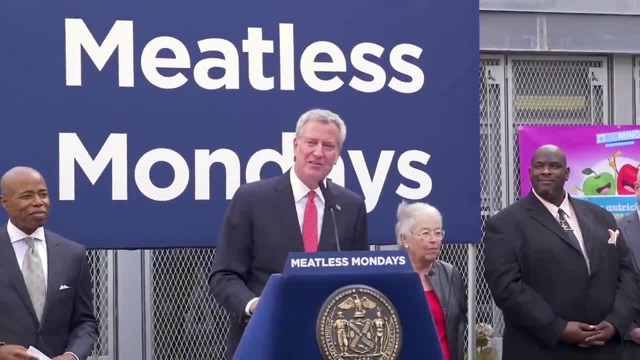 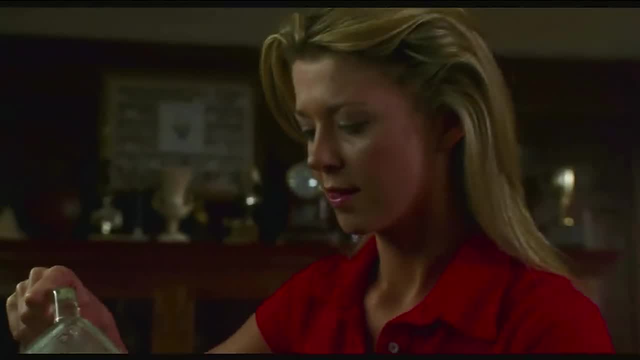 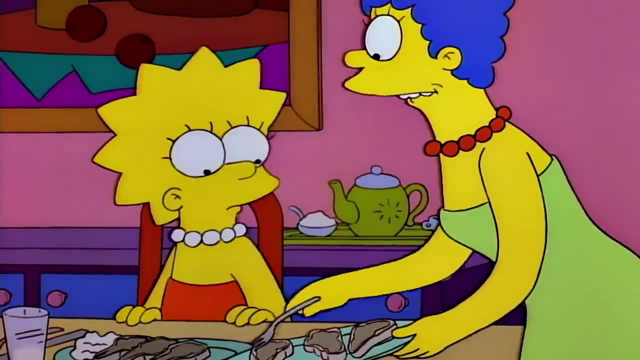 In 15 public schools in Brooklyn we will be instituting Meatless Mondays. Let's hope Mayor de Blasio at least adds an extra soy protein shake to lunch, Especially considering another March 2021 study looking at 187 Polish children found that children not eating meat, a high-quality protein. 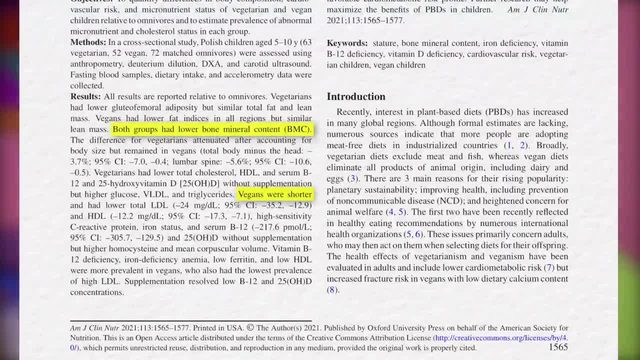 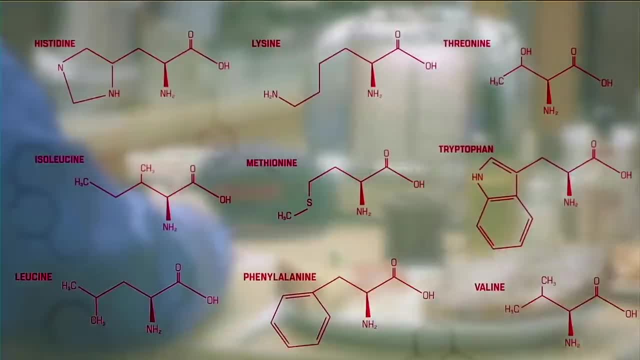 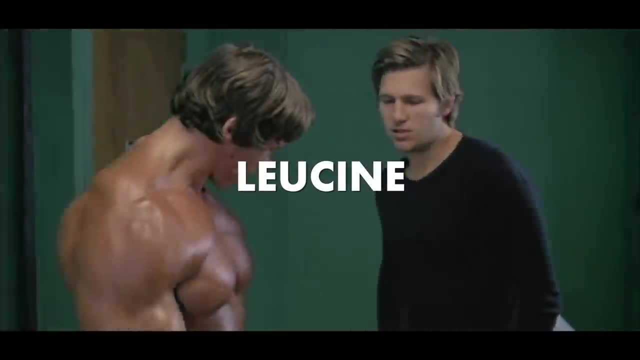 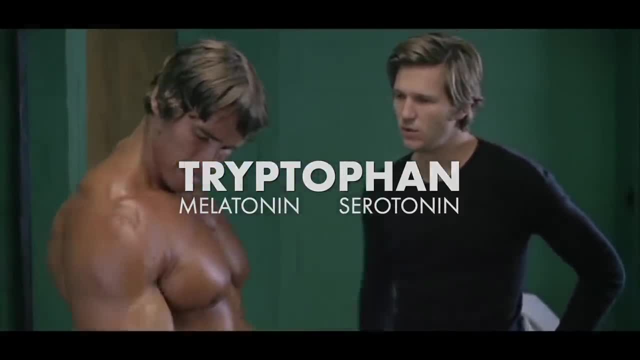 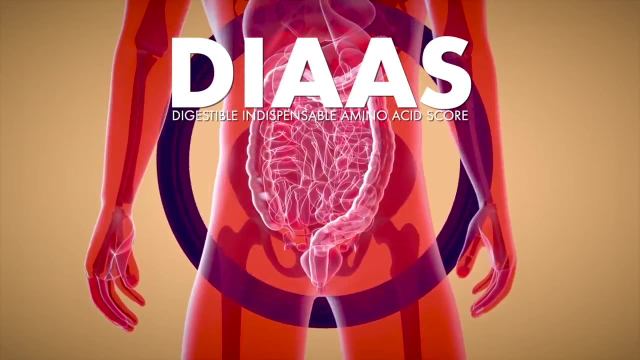 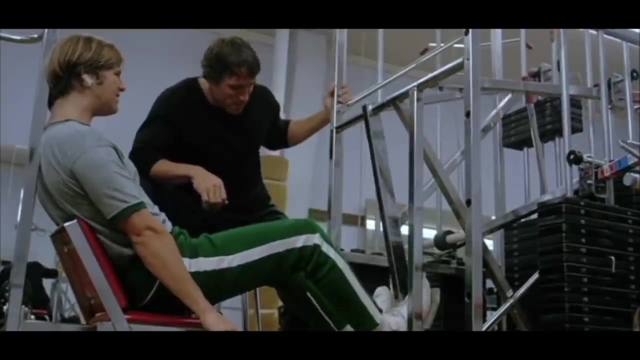 for making the hormones melatonin and serotonin. So DIAZ scores are considering how much and how absorbable the essential amino acids in a food are. Here's an easy example. Say you're trying to gain muscle in the gym. Both leucine and essential amino acid content are important for that. 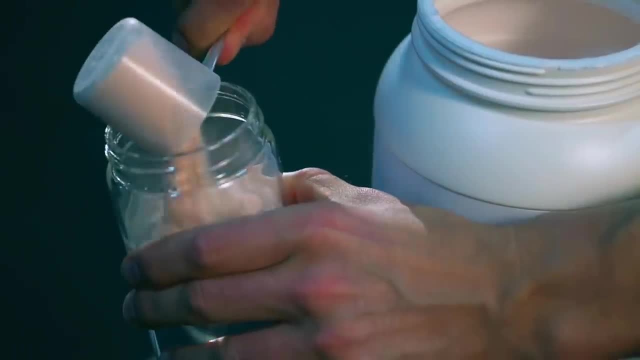 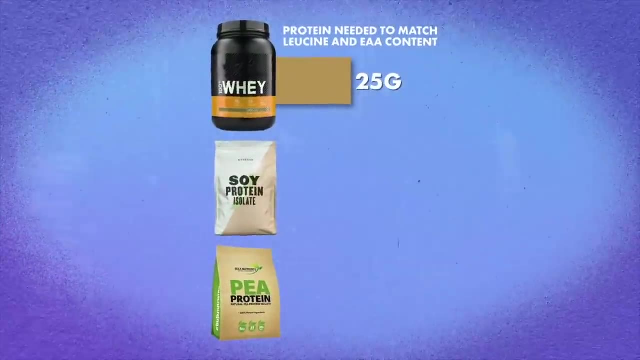 Soy and pea protein powders do have a decent amount of well-digested amino acids, but still to match the leucine content and essential amino acid content of 20% of your body, you'd need 40g of soy protein or 38g of pea protein. This protein quality issue may be why. 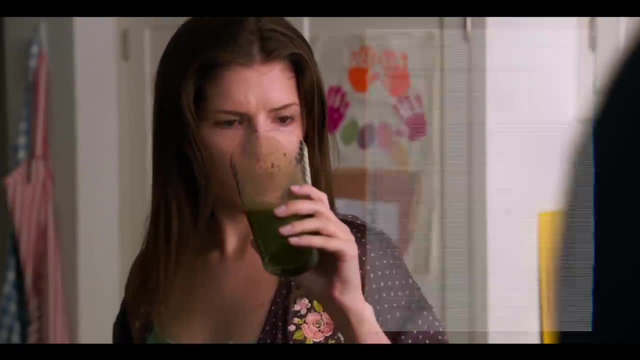 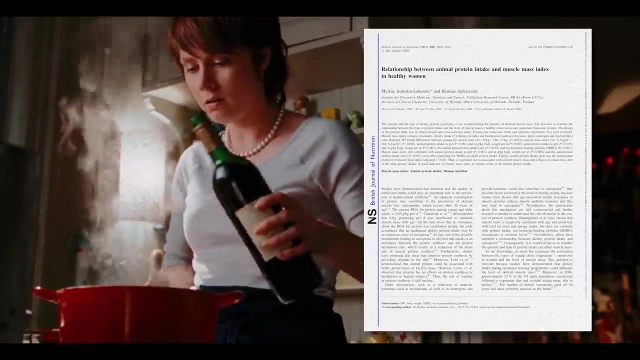 this study found that women not eating meat have less muscle mass than women who do eat meat, even though they ate the same total grams of protein. I ate my 10-15 eggs a day. You know I had my 250g of protein a day But as I got older. 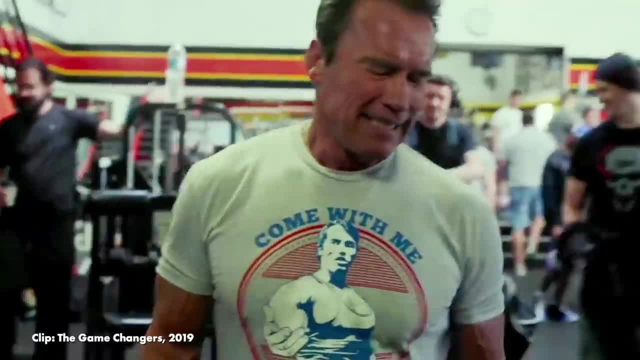 I recognized the fact that you really don't have to get your protein from meat. I ate my 10-15 eggs a day. You know I had my 250g of protein a day, But as I got older I recognized the fact that you really don't have to get your protein from meat. So we started going. 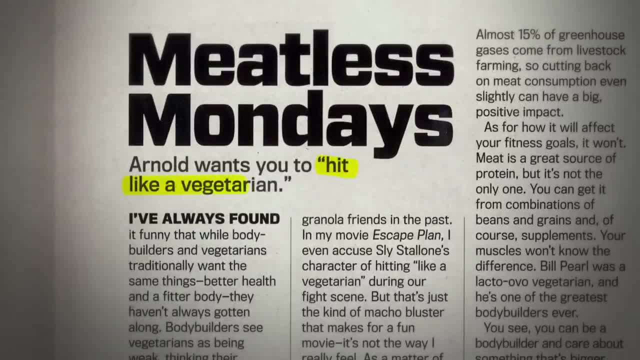 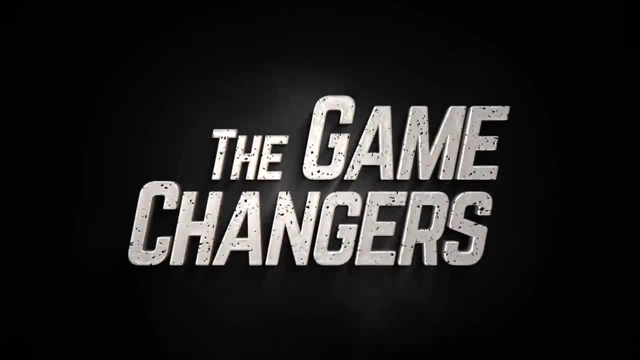 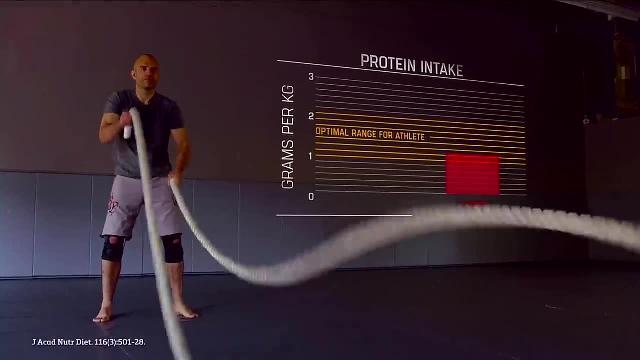 more in the direction of the vegetarian kind of a diet. Of course, plant foods have various benefits other than just protein, but the recent very popular film The Game Changers, backed by big names like Arnold Schwarzenegger and James Cameron, makes it sound like you can get all the protein and the essential amino acids you need from. 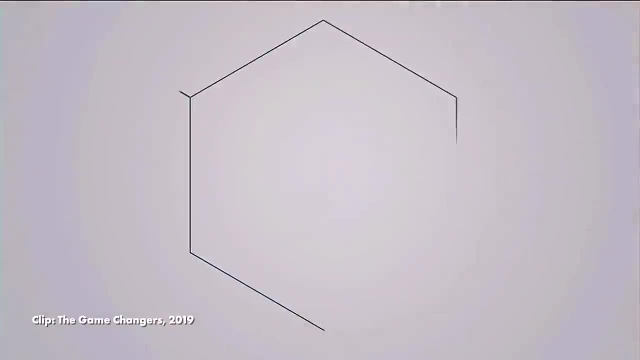 only plant-based foods without much effort at all. For example, one cup of cooked lentils or a peanut butter sandwich has about as much protein as three ounces of beef or three large eggs. Now recent research says the old 50g of protein a day recommendation was way too low. 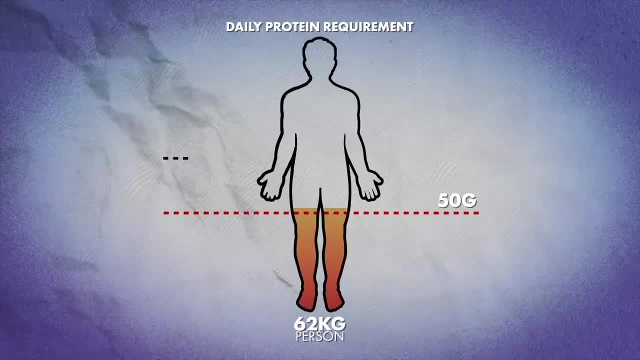 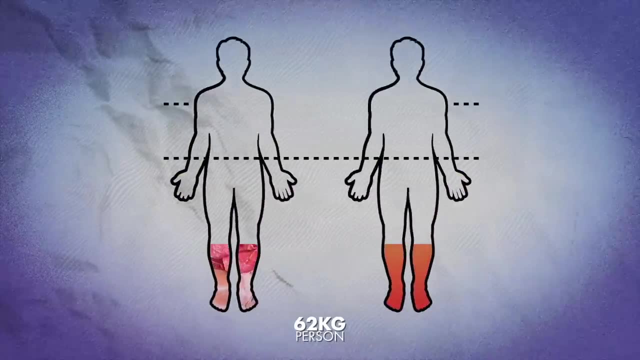 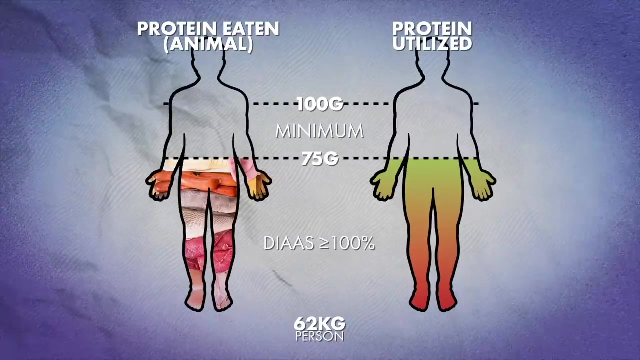 and that a 62kg or 135lb person needs at least 75 to 100g of high-quality protein per day. So if you eat 75g of protein from animal foods, then you've met your protein requirements, because most animal proteins have a DIAS score of 100 or higher. However, since lentils, for example, 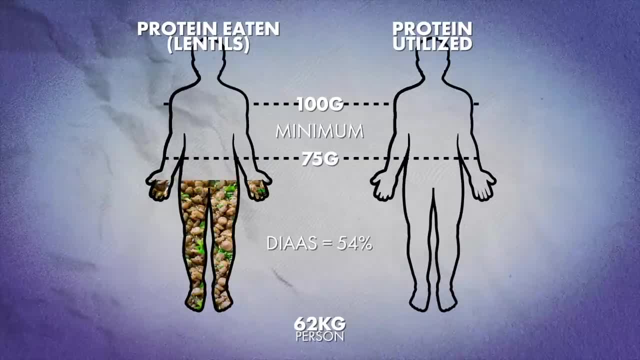 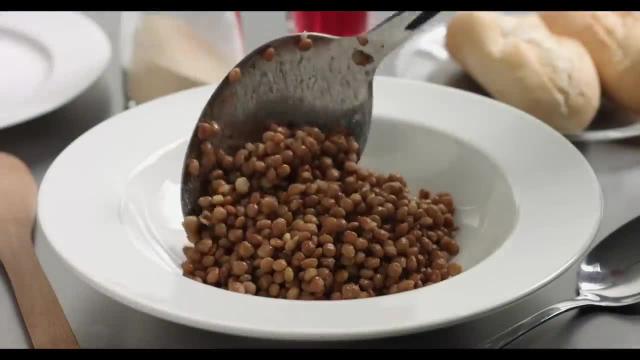 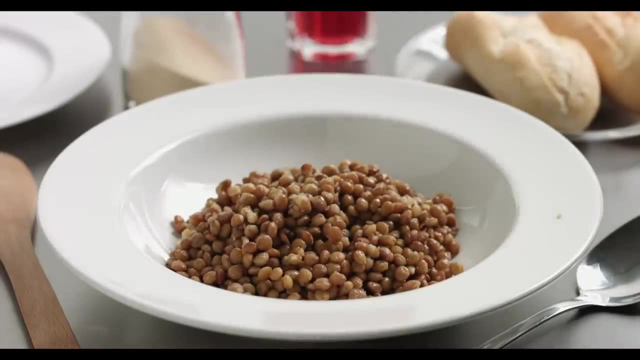 have a DIAS score of only 54,. 75g of protein from lentils would only cover a little over half of your protein requirement. But nobody eats just lentils and you can combine foods to make up for the essential amino acids other foods lack. So it's really good that people typically eat a. 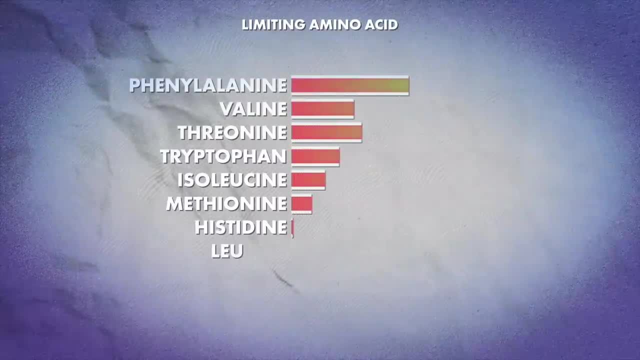 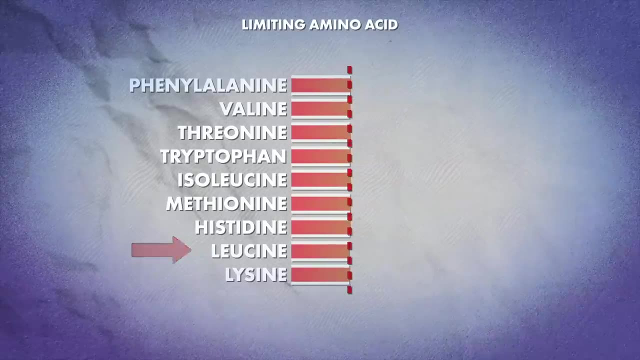 variety of proteins in the same day, because if you're not getting enough of one amino acid, you can't properly utilize the other amino acids. 3. What is the best way to get enough of one amino acid? Cornflakes cereal has a very poor DIAS score of 19, and it is very lacking in the amino acid. 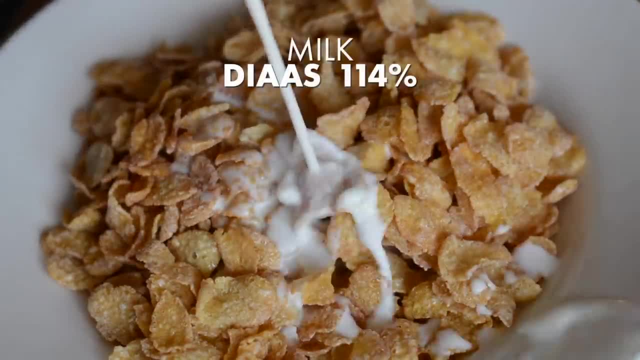 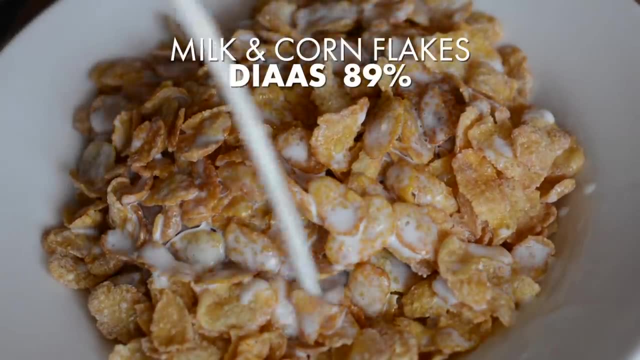 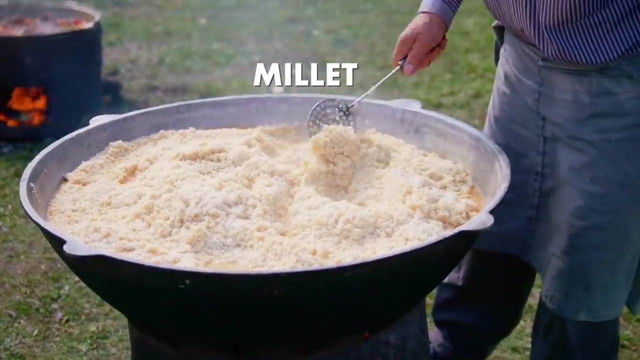 lysine. However, milk has a very high DIAS score of 114, and has plenty of extra lysine. so if you eat your cornflakes cereal with milk, like most people do, then the DIAS of your breakfast is actually 89.. Also, eating lentils with your millet will improve the protein quality of the millet. 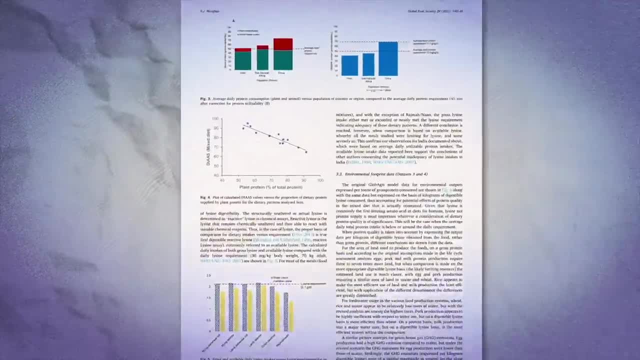 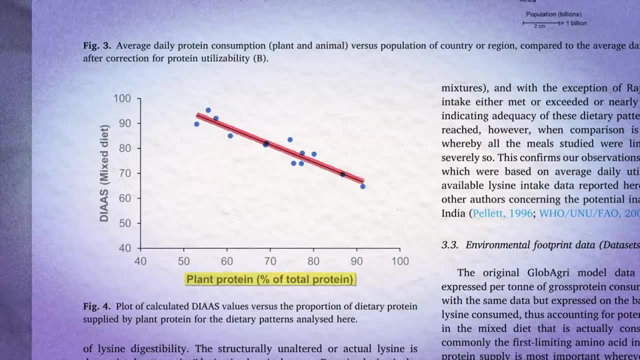 But unfortunately, as this 2021 paper shows, as the percentage of plant protein in the diet goes up, the overall protein quality of the diet goes down. In this study, even athletes who were following a vegetarian diet didn't end up getting the 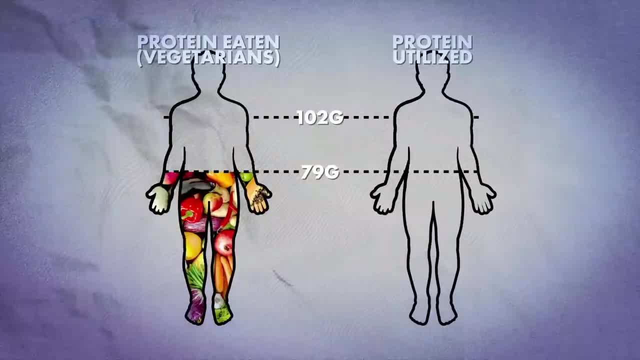 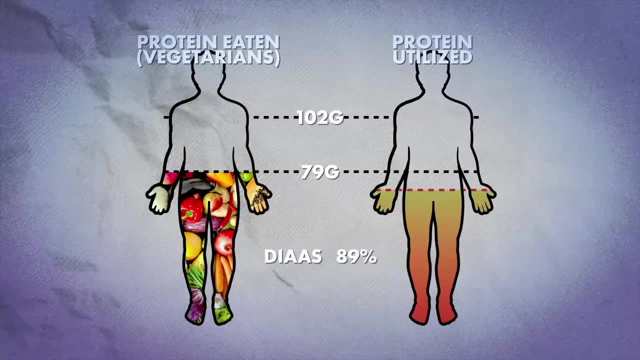 minimum recommended amount of protein. The vegetarian athletes were getting enough protein in terms of total protein, but they only utilized 89% of the protein they ate, so they missed the lower end of their protein target by 10 grams and the upper end of the. 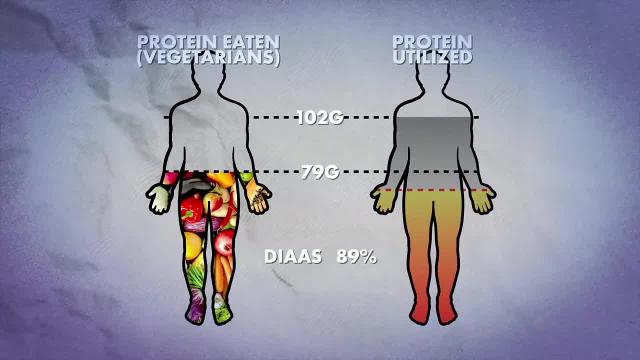 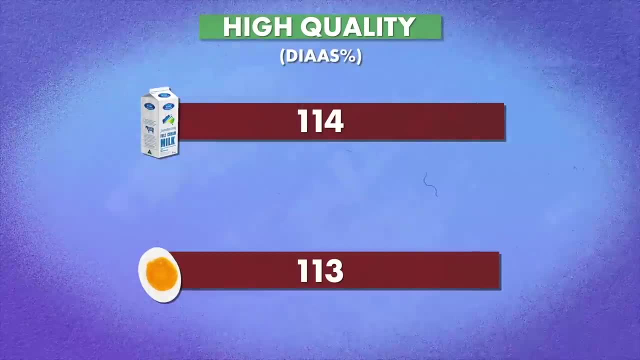 target by 22 grams of utilizable protein. Now, 89% is actually not bad, but as vegetarian, they would be eating high-quality proteins like dairy or eggs. so if they were vegan, we would expect their overall protein to be a lot lower than 89% utilizable. 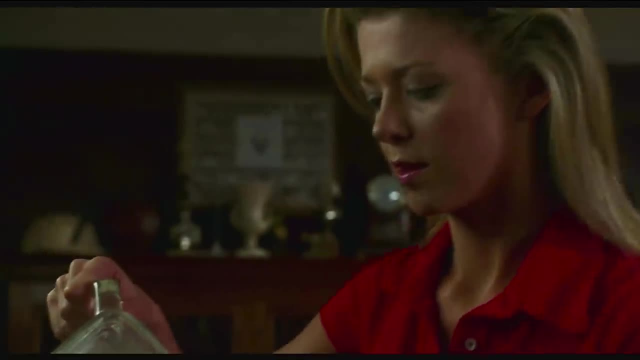 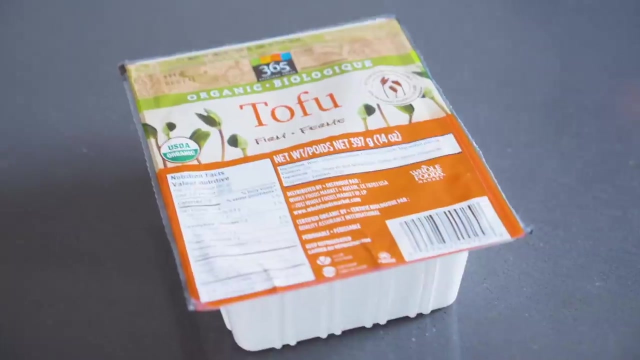 The solution for these athletes is quite simple really. they could just add another scoop of soy protein powder a day. But it was surprising to me that even these athletes, who I imagine would be very calculated with their protein, could be missing the recommended protein intake. 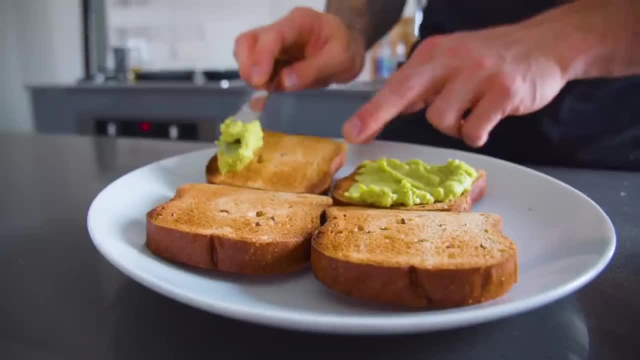 With the right knowledge and diligence. yes, you can meet your protein requirements on a vegetarian or vegan diet. But if you are a vegetarian, you might want to go for a vegan diet. But if you are a vegetarian, you like it. but you need to make sure to pick the right proteins. 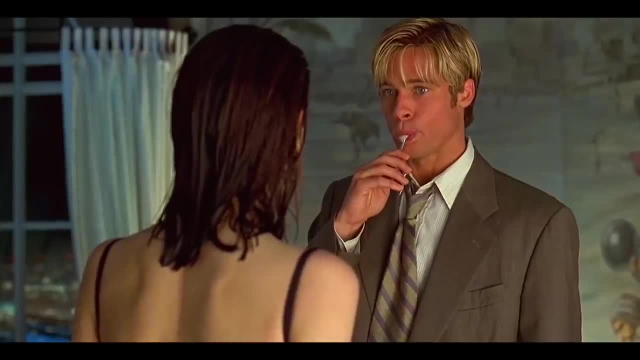 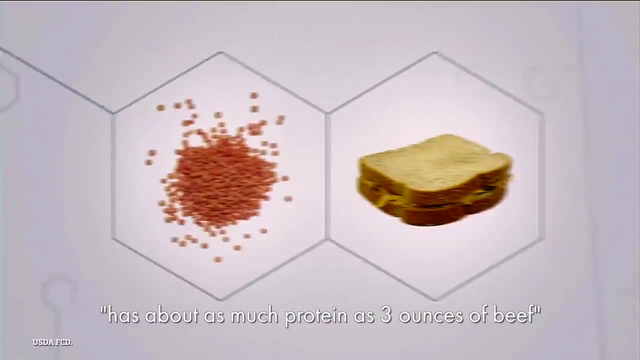 What are you eating? You can't buy it. Let's go back to this example from the game changers: 1 cup of cooked lentils or a peanut butter sandwich has about as much protein as 3 ounces of beef or 3 large eggs. 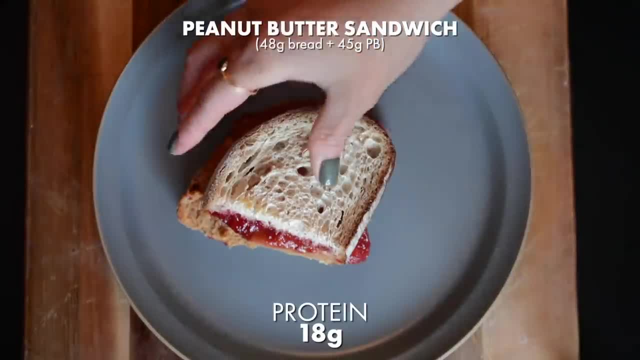 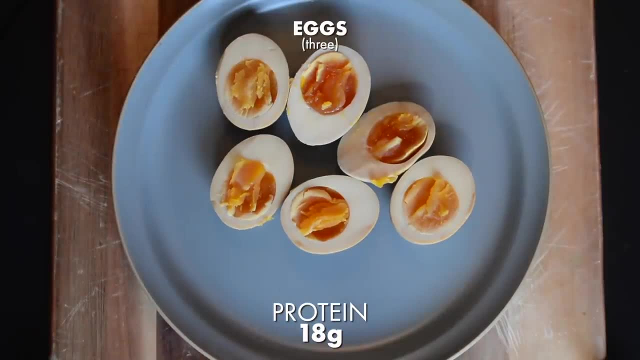 So yeah, technically you get the same grams of crude protein from a peanut butter sandwich, a cup of lentils, a 3 ounce steak or 3 eggs. But let's look a little closer. Here are the dyascores of an individual's protein intake. The protein intake is always different than the. 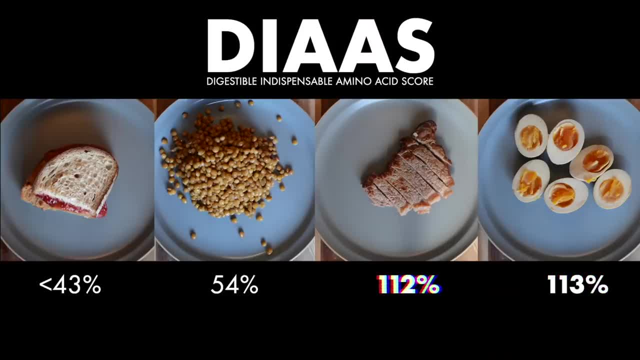 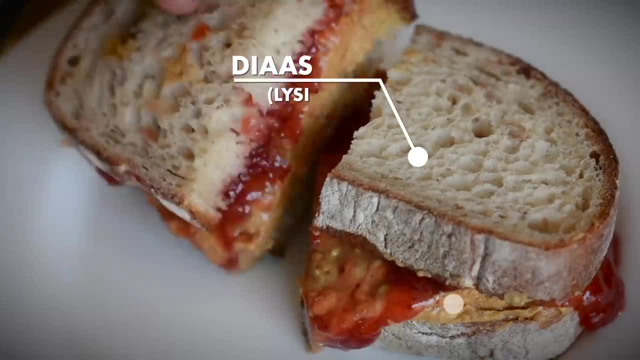 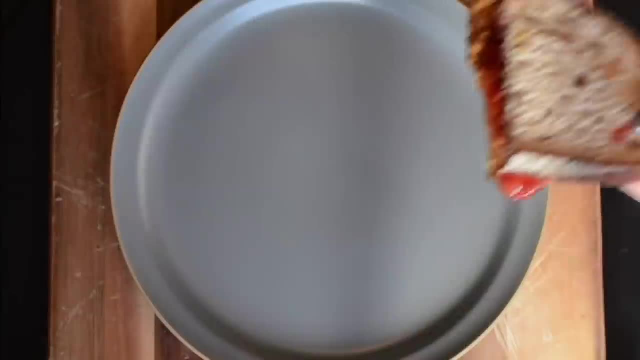 these foods: Boiled eggs are 113, beef is 112, lentils are 54, roasted peanuts are 43 and wheat bread is 29.. Wheat and peanuts are both limiting in lysine, so even if you combine them, their dia score couldn't be higher than 43.. So let's say you start off with a peanut butter sandwich. 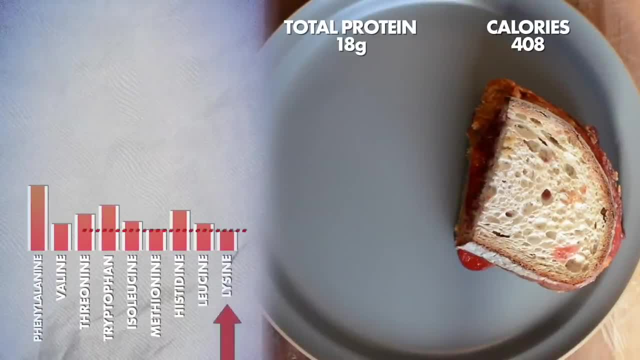 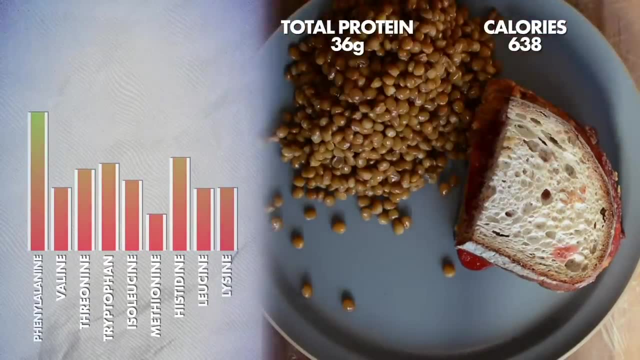 Here's the amino acids you're getting. So we'll want to make up for the poor lysine content of the peanut butter sandwich. So you can add some lentils which have plenty of lysine and this will have increased the overall protein quality of the meal. But now you're still quite low in methionine. 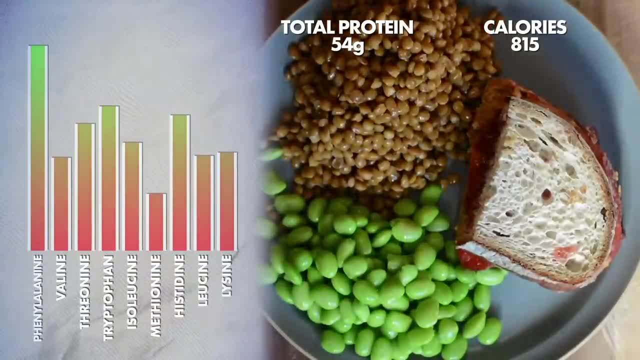 So then you add some edamame boiled soybeans because they're one of the best plant sources of methionine, But even then you're not getting that much methionine relative to all the other amino acids. So that's the amino acids you're getting from 54 grams of protein from these plant. 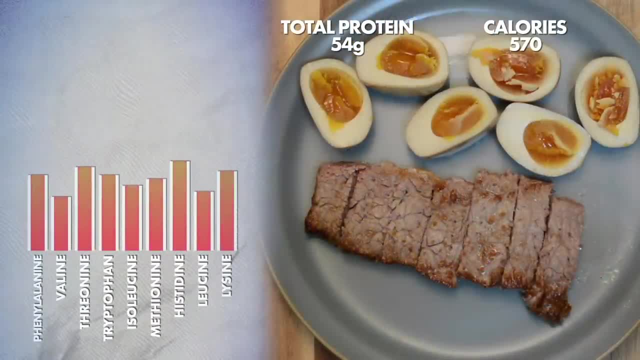 foods. Now compare this to what you get from just eating three eggs and a four and a half ounce skirt steak. Well, at first glance you can see that there's a lot of protein in the meal. But if you add a little bit more protein to the meal, 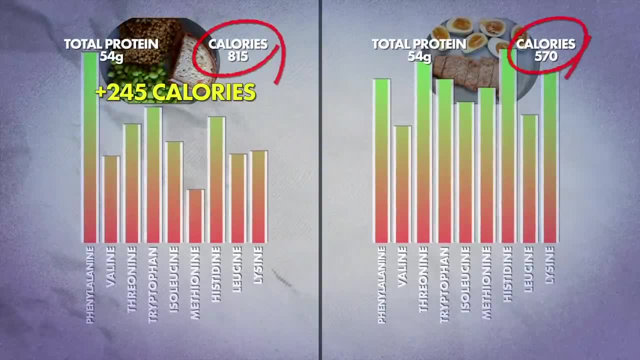 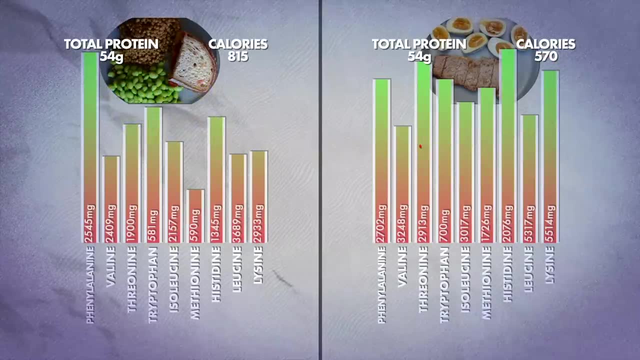 you can see that with a plant-based meal, you have to eat 245 more calories to get less essential amino acids And you get a better balance of the amino acids from the animal proteins. So the point is, if you're not eating meat, you'll need to get a variety of plant proteins every day. 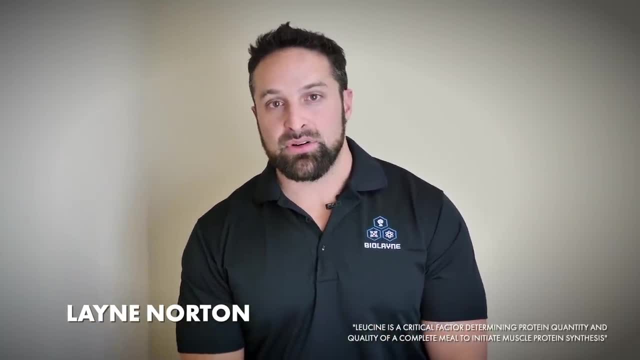 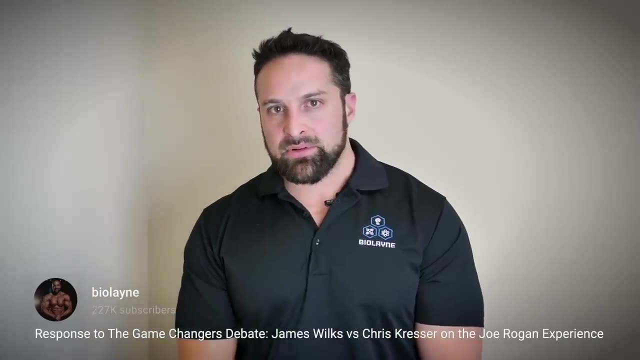 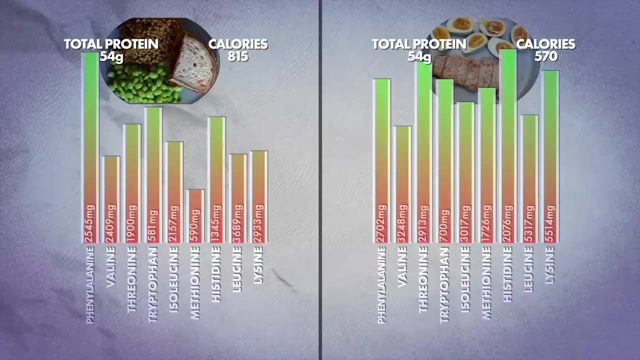 Dr Lane Norton did his PhD dissertation on the critical role of the essential amino acid leucine in building muscle. He discussed in this video here how, despite the game changers being all about athletes and performance, it glossed over this very important topic. So, with 54 grams of protein from steak and eggs, 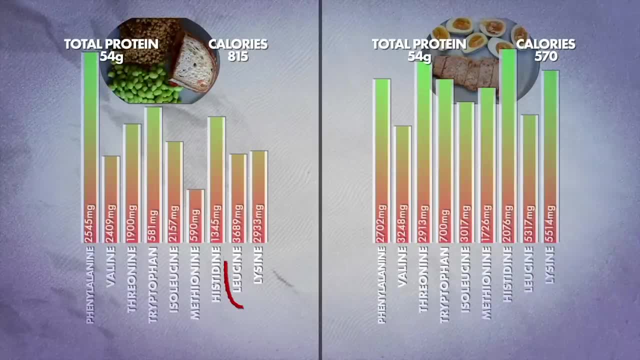 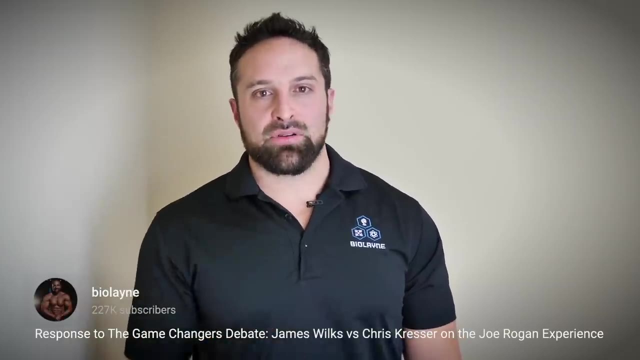 you're getting 5.3 grams of leucine but only 3.7 grams from the plant-based meal, Meaning you'd have to eat almost 1200 calories of these plant foods to match the leucine content of the steak and eggs meal, which is only 570 calories. You can get enough protein from. 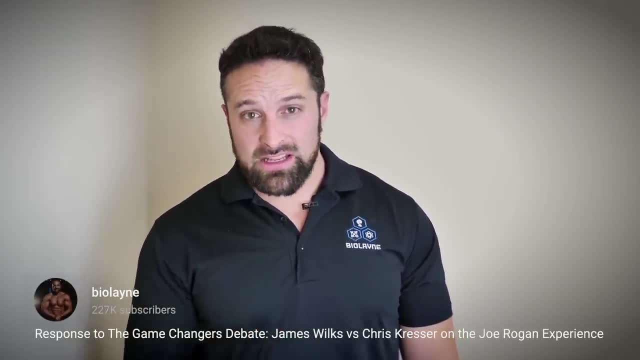 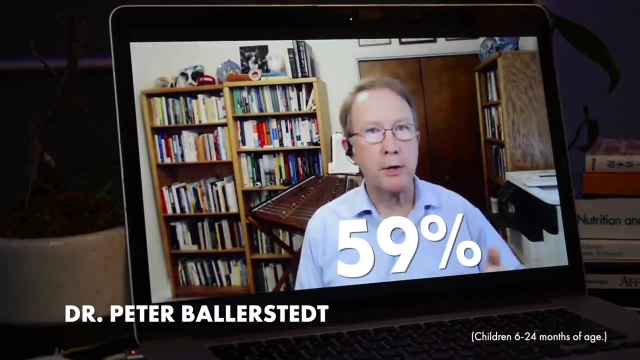 vegan sources of protein. but if you're using a whole food vegan source of protein, you are going to have to eat a ton of them, Something like 59% of children globally doing global food Aren't given eggs, seafood, dairy and meat. 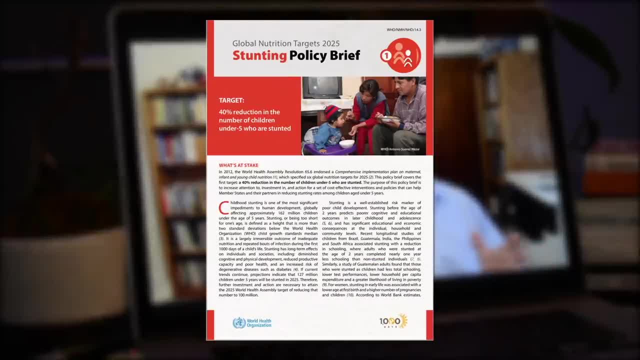 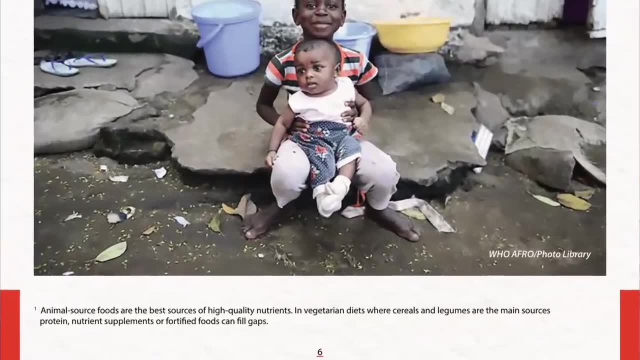 And the WHO says the best foods for them are the meat-eggs-dairy-seafood. Now they say it in a footnote. In the text they say high-quality right or nutrient dense or something like that, but down in the footnote they specify: i had a chat with forage agronomist and animal nutritionist. 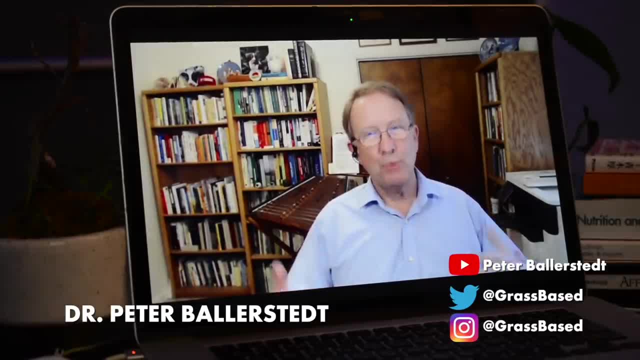 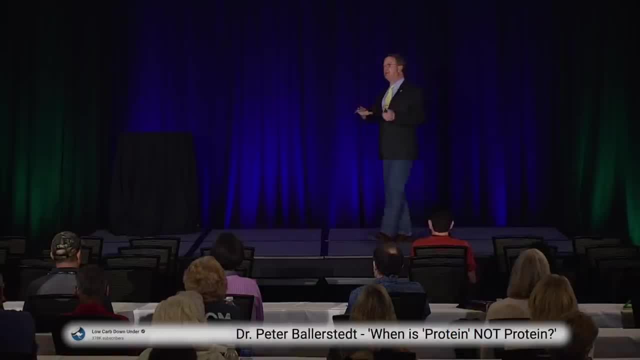 dr peter ballersted, who has been a key voice on this protein quality topic. in fact, his detailed presentation on youtube called when is protein, not protein, is what got me interested in this topic. in that presentation he gets into a lot of important nuances, for example, processing plant. 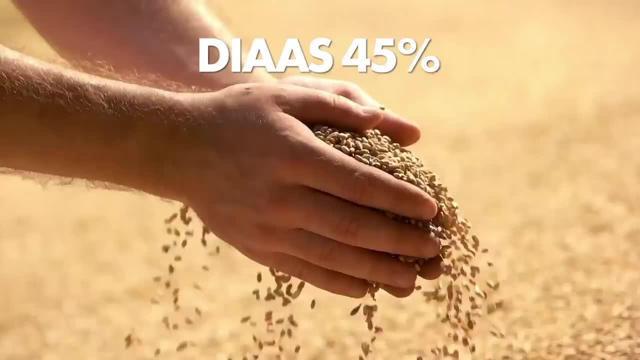 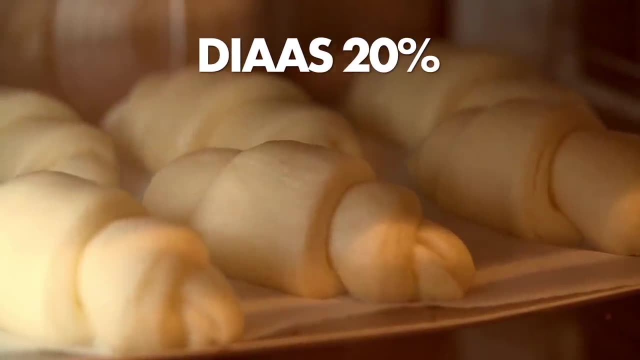 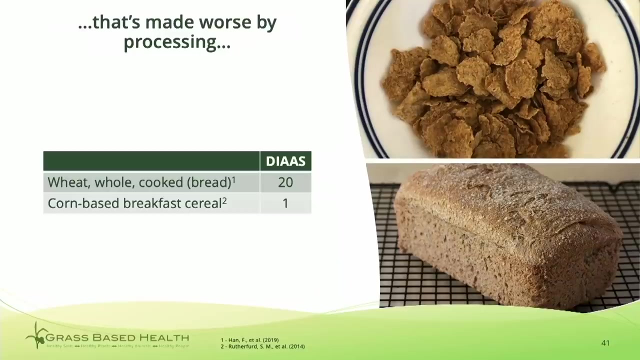 foods can lower the protein quality of that plant food. for example, we don't just eat wheat, we process that wheat into bread and that processing actually worsens the protein quality, and so we make whole wheat bread. we cut that value in half because all this processing inactivates, makes unavailable the 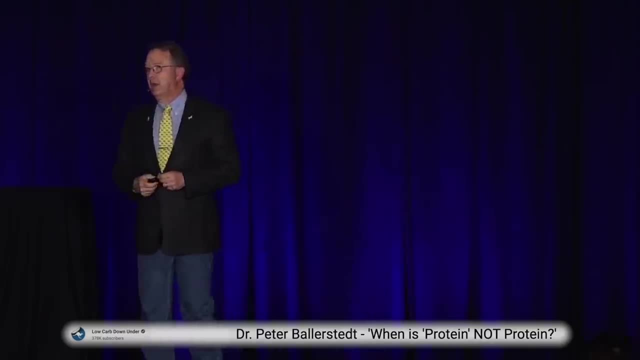 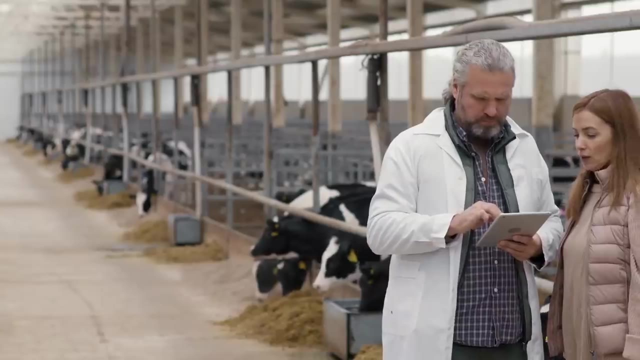 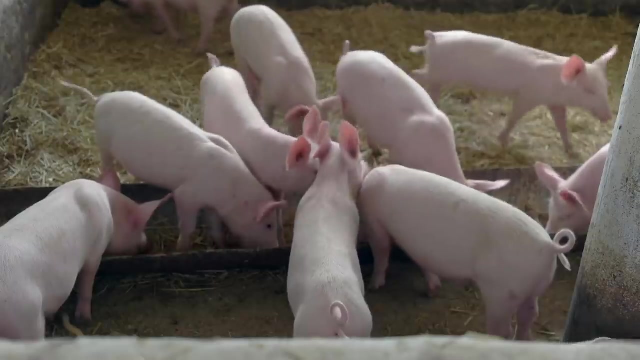 lysine, which is already the limiting nutrient. interestingly, human nutritionists don't fuss too much about protein quality or specific amino acids. but for an animal nutritionist like dr ballersted, paying attention to protein quality is just complicated common sense. after all, animal nutritionists have been balancing the rations given to pigs based not 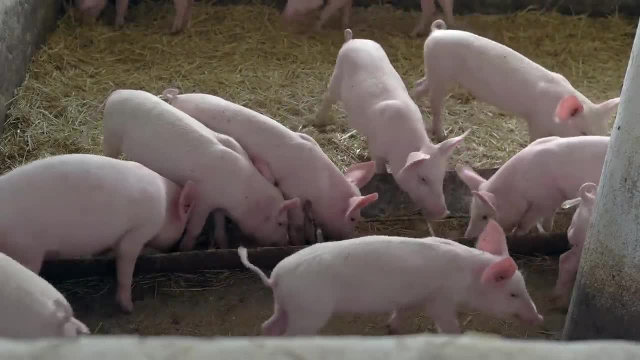 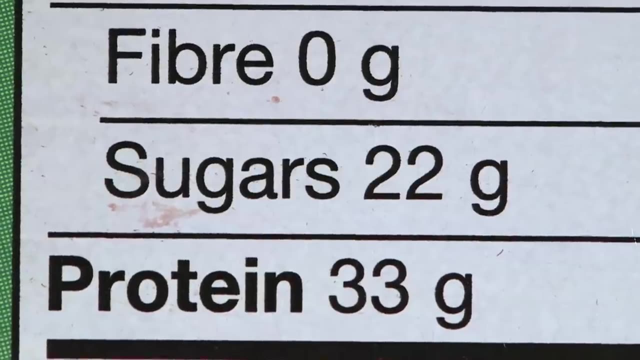 just on protein, but amino acids. for almost 40 years now, in fact, the fao has suggested that maybe we should be putting individual amino acids on food nutrient labels. this protein quality discussion is important not just because of the recent popularity of plant-based diets, but also. 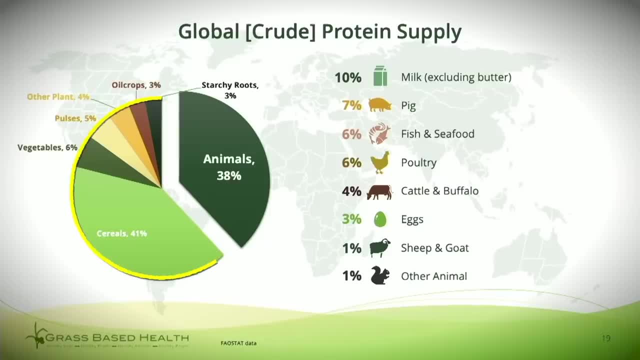 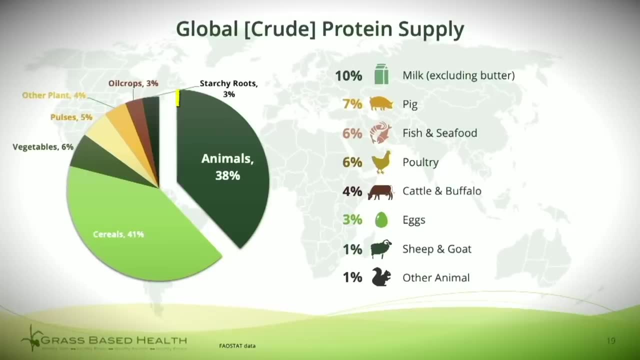 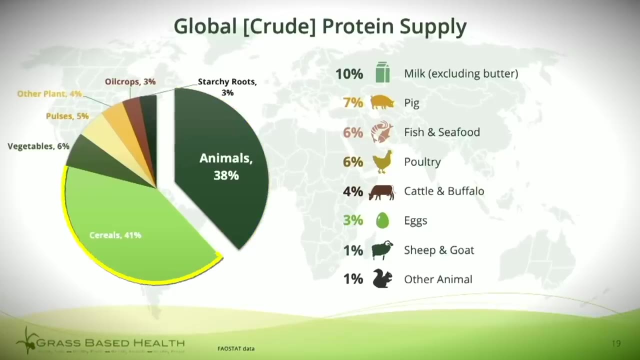 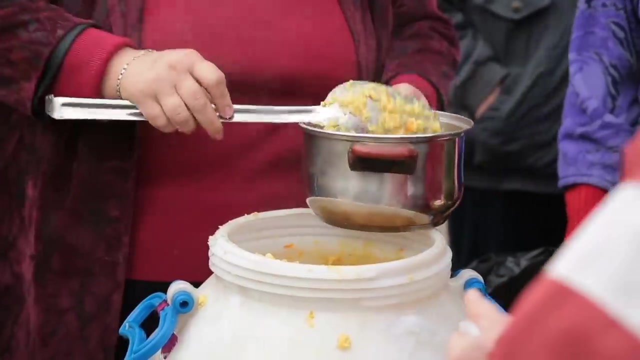 as dr ballersted points out, more than 60 percent of our current global protein supply is already plant-based, so humanity gets less of its protein supply from all animal source foods combined than it does from cereals. now, developed countries certainly eat much more animal source foods, so you might be thinking protein quality is an issue for developing. 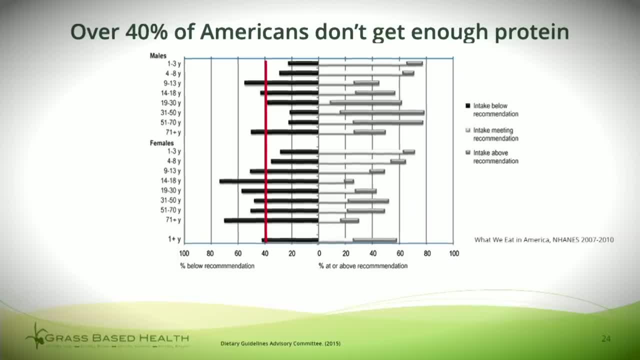 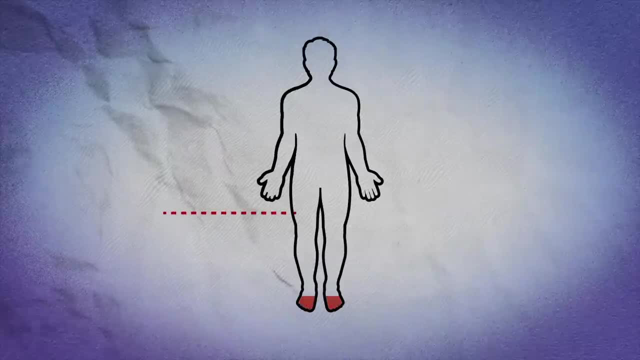 countries well, as mentioned earlier, data from 2015 says forty percent of americans are not getting the minimum recommended amount of protein and that is based on the old low recommendation Cornelius Nelson whole plants does do is helpful for towns with large, and that is based on the old low recommendation of 0.8 grams of protein per kilogram body weight.